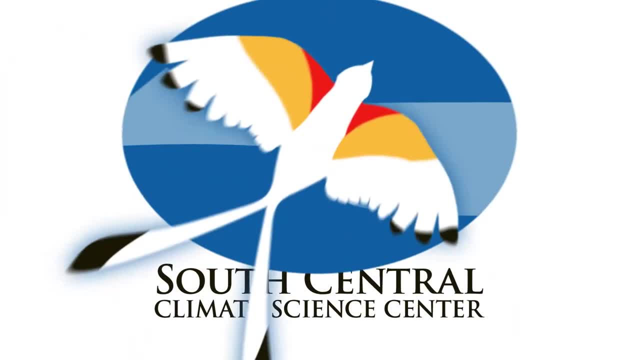 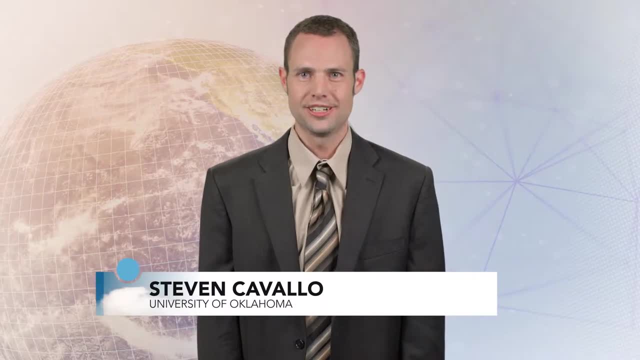 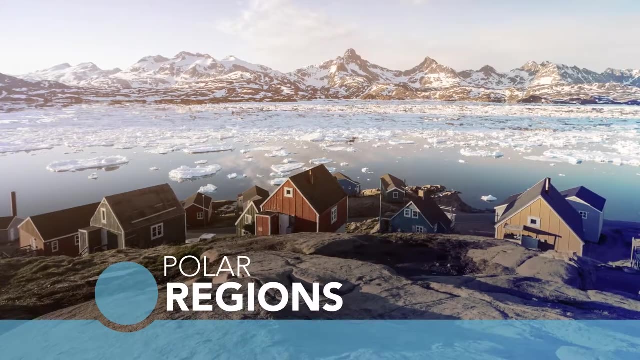 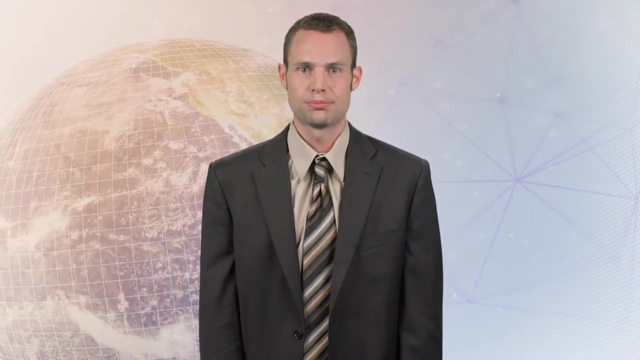 Hello, I'm Dr Stephen Cavallo, Associate Professor at the University of Oklahoma School of Meteorology. In this video, I'll be discussing impacts of climate change in polar regions. The impacts of a changing climate on the polar regions are profound. In part, this is because 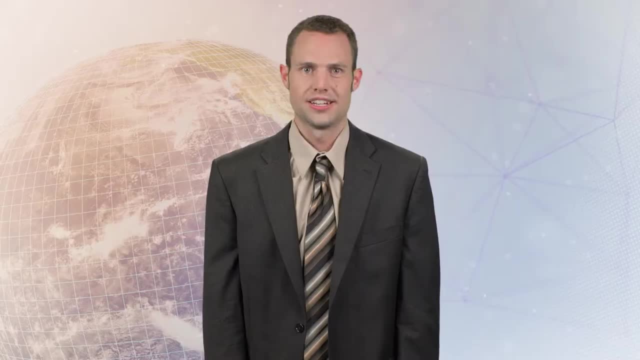 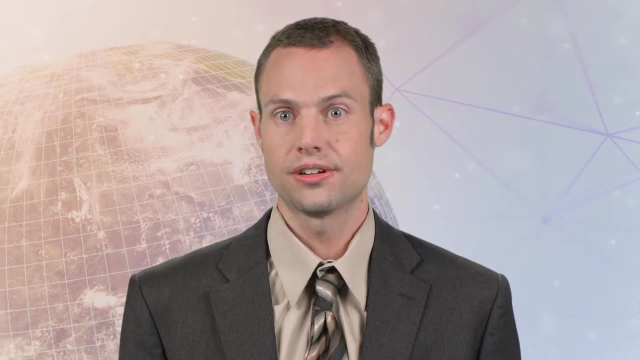 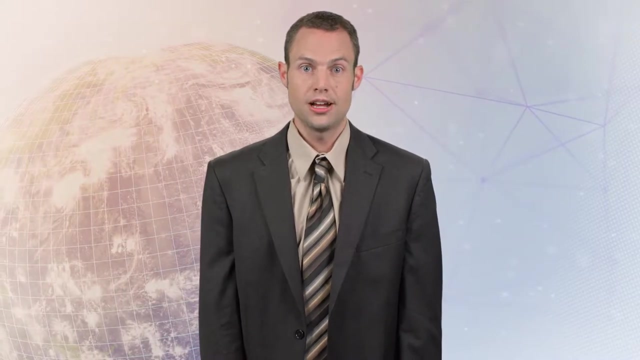 the Arctic is warming faster than anywhere else on Earth. As global temperatures rise, not every part of the globe will warm equally. Differences in warming can arise when components of the Earth's system interact with each other, causing the warming to speed up or slow down. In the Arctic, the warming is sped up by an interaction between ice and ocean. 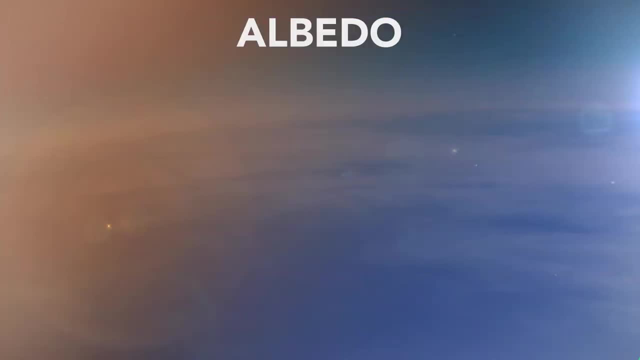 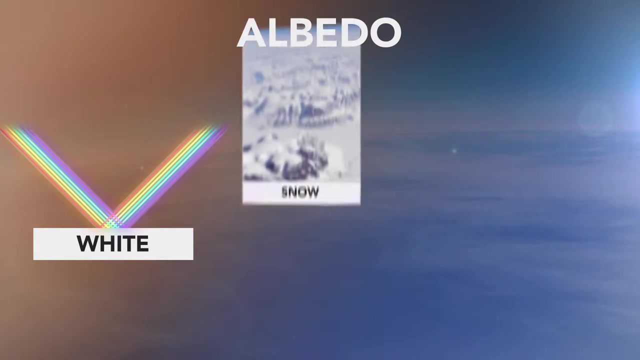 that we call the ice albedo effect. The albedo of an object describes how much of the sun's radiation the object reflects back into the atmosphere. For instance, when we see color, what we are observing is how much light is reflected or absorbed by an object. White surfaces are highly reflective. This includes surfaces. 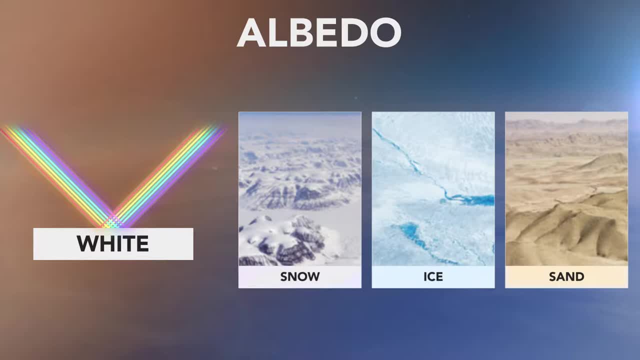 such as snow, ice or sand. On a sunny day, when you're walking along a sandy beach or driving down a snowy road, you'll probably need sunglasses due to the high amounts of sunlight being reflected. In contrast, dark surfaces are not very reflective, such as 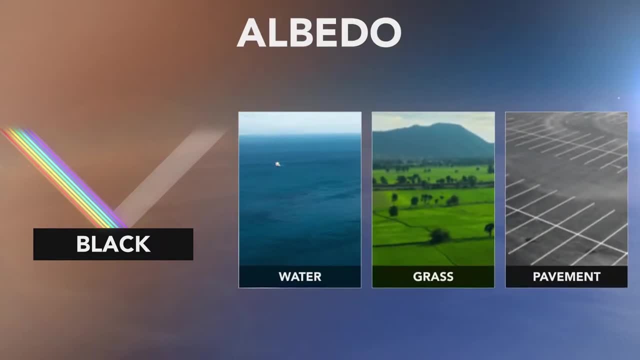 water, grass or black pavement. You wouldn't want to walk barefoot on black pavement on a hot summer day, because this surface is absorbing just about all of the radiation that hits it instead of reflecting it, making it very hot. Ocean water absorbs about 94%. 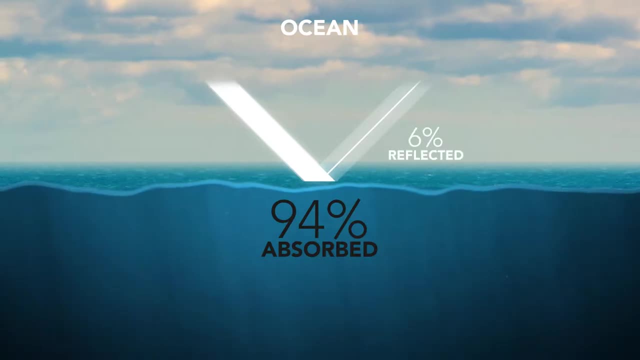 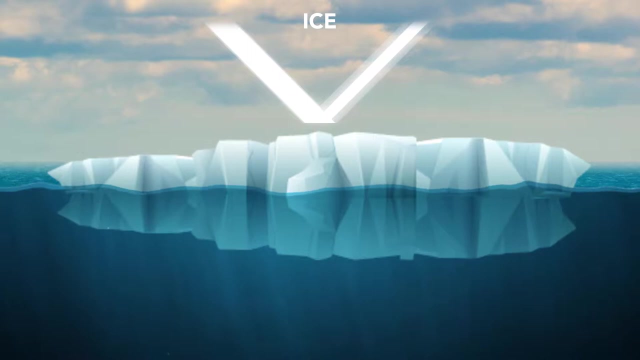 of the sun's incoming radiation, while only 6% of the sun's radiation is reflected back up to the atmosphere. Ice, on the other hand, is much more reflective. Sea ice reflects about half of the sun's radiation, and thus only half of the sun's radiation is absorbed. 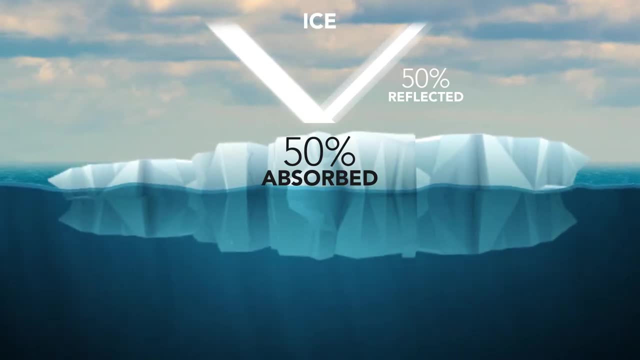 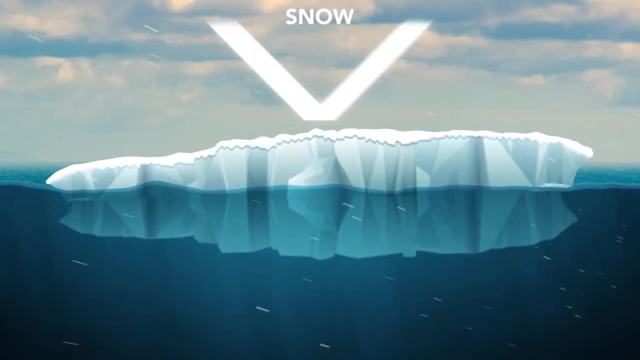 into the ocean. So when the ocean is topped with sea ice, the ocean does not warm very efficiently. Snow is even more reflective than ice, So when sea ice has snow on top of it, which it usually does, it reflects about 90% of the sun's radiation, leaving 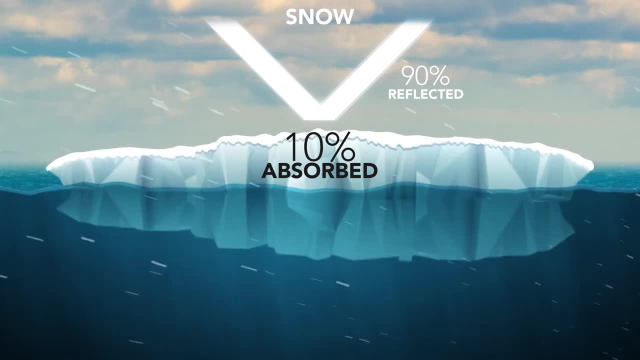 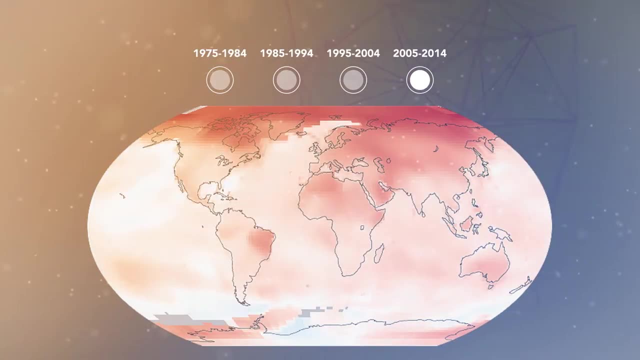 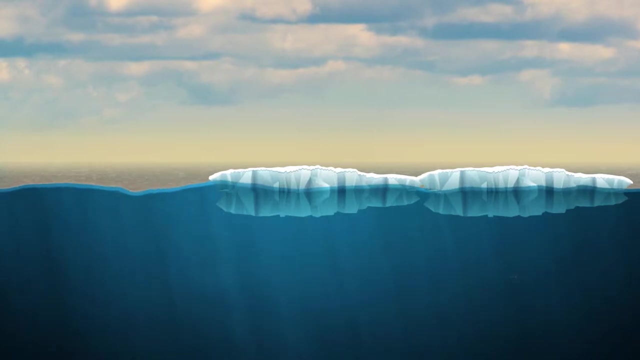 only 10% to be absorbed into the ocean, So in this case it's very difficult to heat the ocean. However, rising surface temperatures are causing sea ice formations to melt. As the ice melts due to warming surface temperatures, a larger percentage of the ocean is exposed. 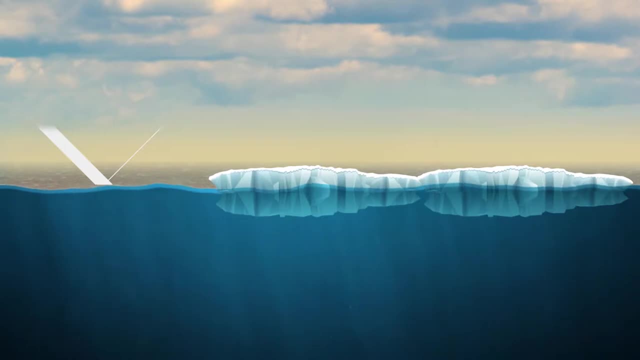 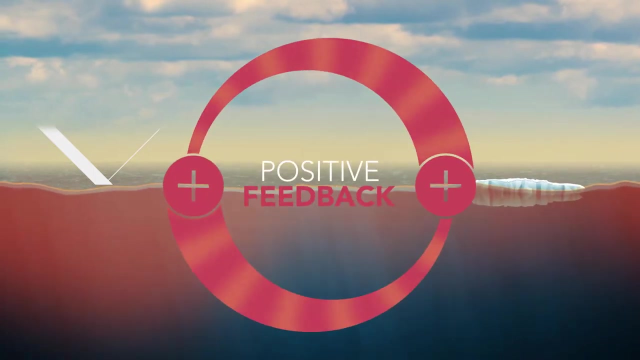 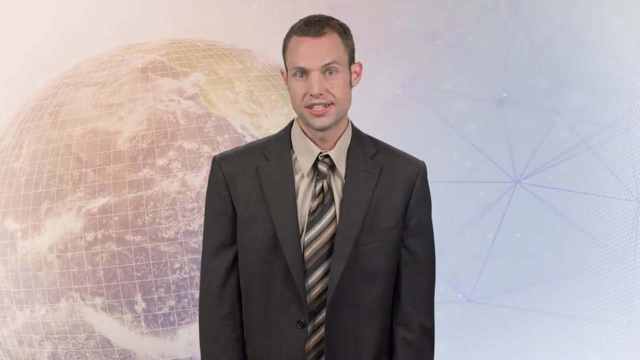 because the ocean has a lower albedo than ice, the ocean begins to warm. This ocean warming in turn causes the sea ice on top of it to melt even faster. This is an example of a positive feedback loop. We can see the observed effect of the ice albedo positive. 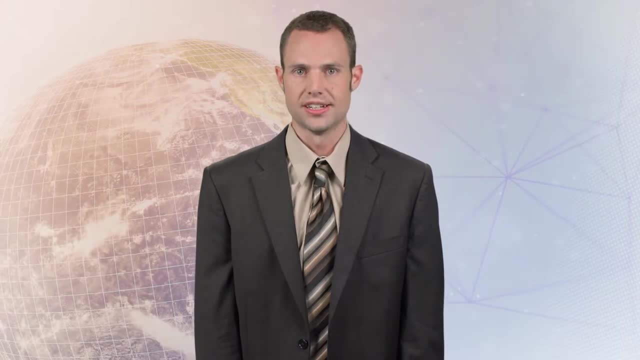 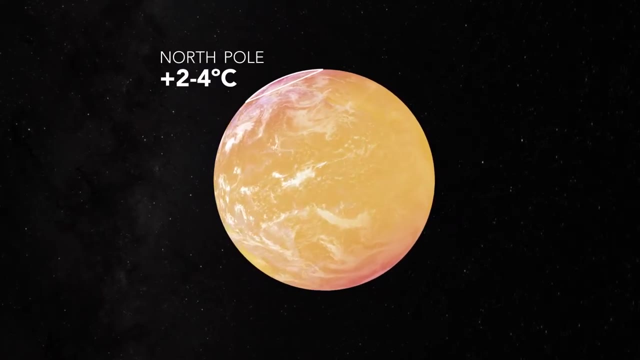 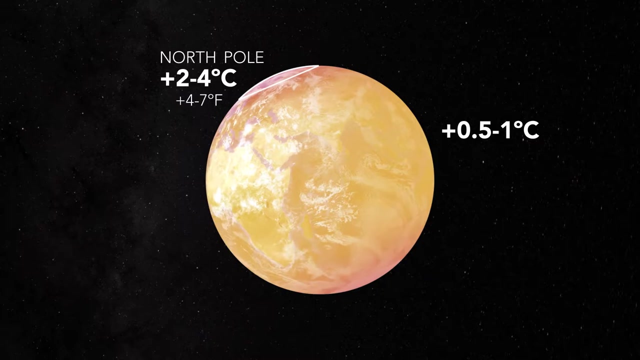 feedback loop in global temperature trends from 1981 to now. Notice that temperatures have warmed more over the Arctic sea ice regions about 2-4 degrees Celsius or about 4-7 degrees Fahrenheit, in comparison to elsewhere across the globe where it's about 0.5 to 1 degrees. 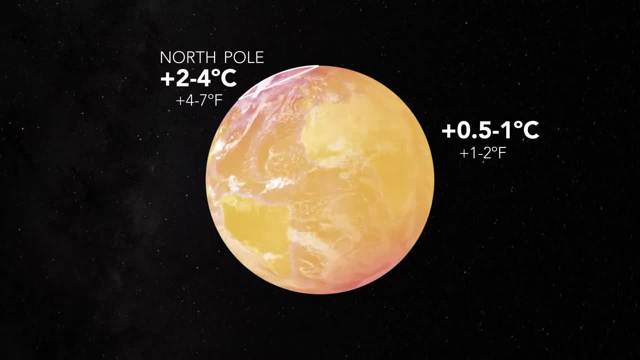 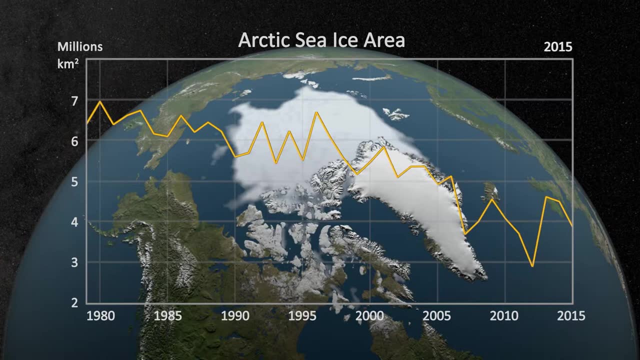 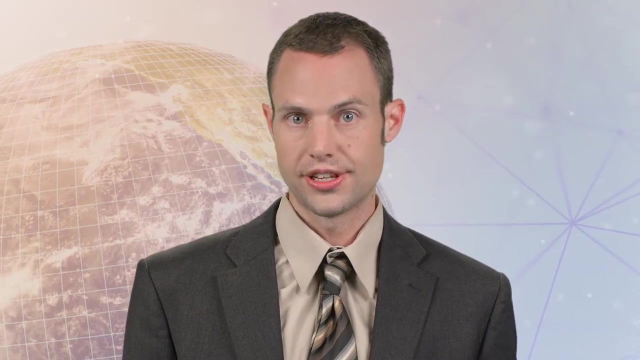 Celsius, or 1 to 2 degrees Fahrenheit. This animation from NASA illustrates the accelerating loss in Arctic sea ice that is occurring primarily from this feedback loop. We don't observe this same positive feedback loop, however, over the Antarctic. This is because, in order for this positive feedback loop to begin, temperatures have 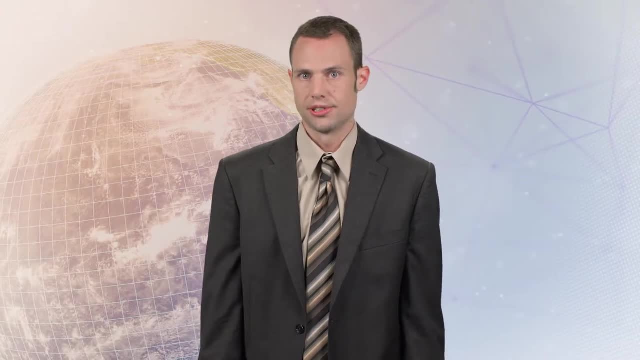 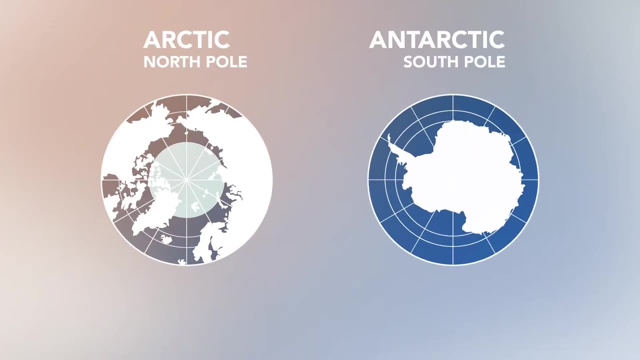 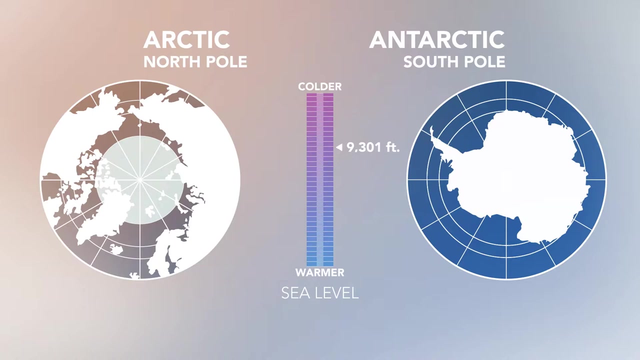 to warm to the point where water turns from solid into a liquid, which is 32 degrees Fahrenheit or 0 degrees Celsius. The Arctic is usually warmer than the Antarctic because the elevation is generally lower. The South Pole, for example, is located at 9,301 feet above sea level, while the North 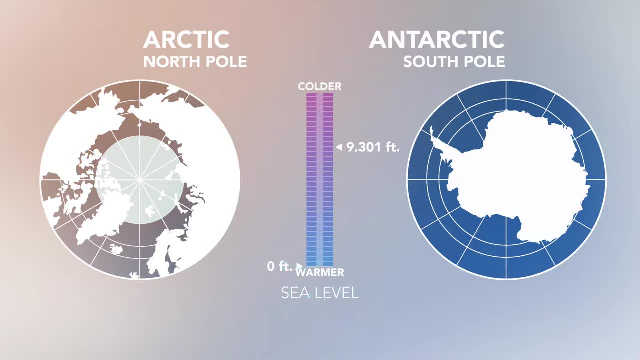 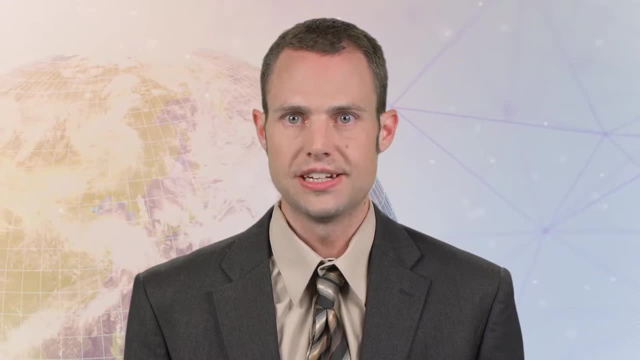 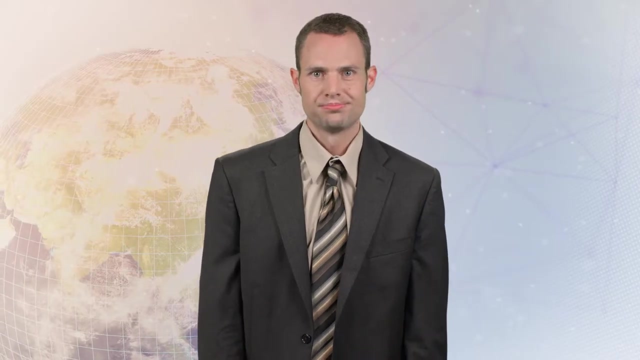 Pole is at sea level. This keeps temperatures well below freezing at the South Pole all year round. However, as temperatures continue to rise, we are starting to see this feedback in some of the areas of Antarctica where temperatures are warmest. So you may have heard that melting sea ice contributes to sea level rise, but this isn't. 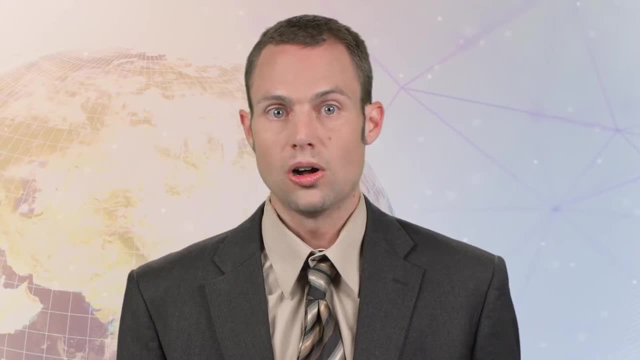 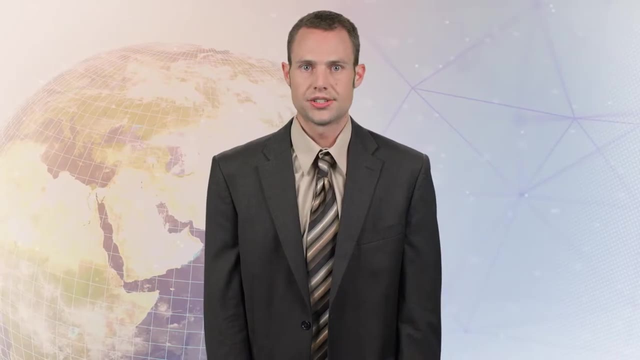 the case. In fact, if all of the sea ice in the Arctic Ocean melted, there would be no significant increase in global sea levels. This is because all the mass of the ice is already in the ocean, so the total mass will not change. 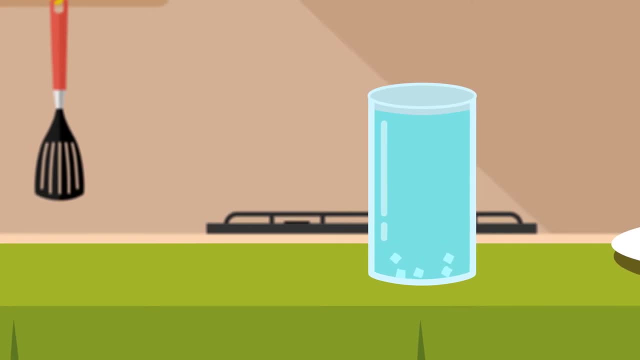 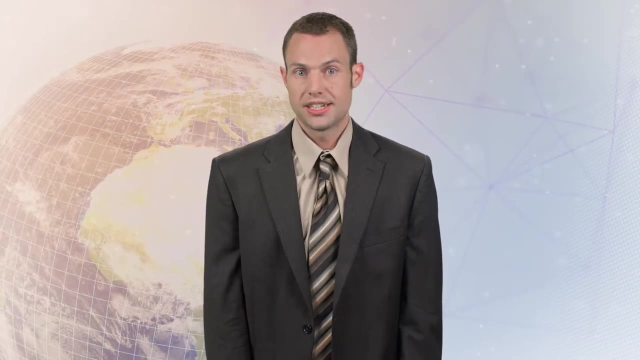 You can observe this same effect when you notice that your iced water is now as cold does not overflow when the ice melts. What does contribute to sea level rise is the melting of ice that currently sits on land rather than ocean. Your iced water would certainly overflow. 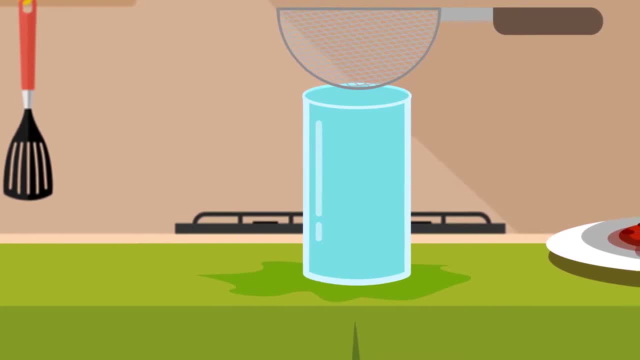 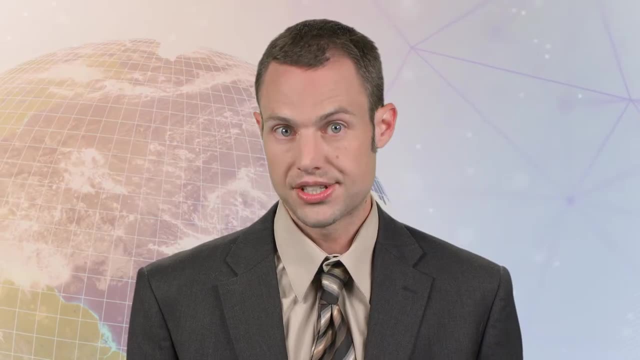 if you let melting ice cubes from outside of your cup drain into it. If the land ice that sits on top of Greenland breaks away and falls into the ocean, this will cause sea levels to rise substantially, because entirely new mass is being introduced to the ocean system. 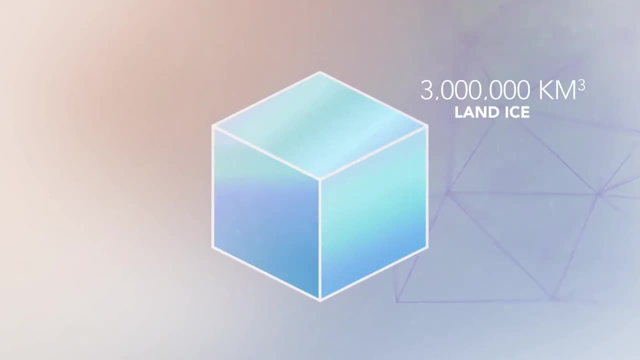 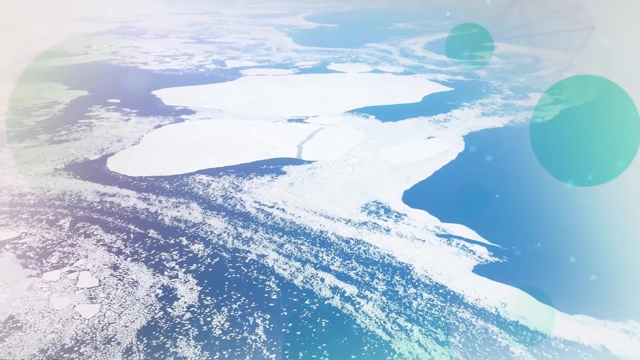 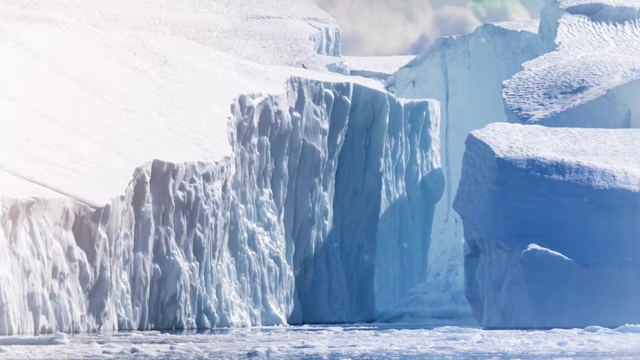 There's an estimated 3 million cubic kilometers of land ice on Earth, and that has already begun to melt into the ocean. The warming temperatures are already leading to Greenland ice melt each summer. If the entire Greenland ice sheet were to melt, it would raise sea levels by an average of seven meters. 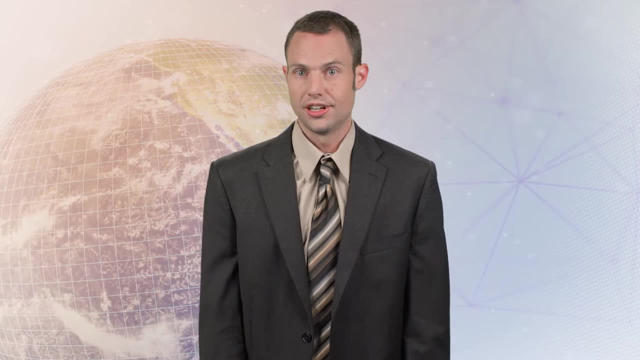 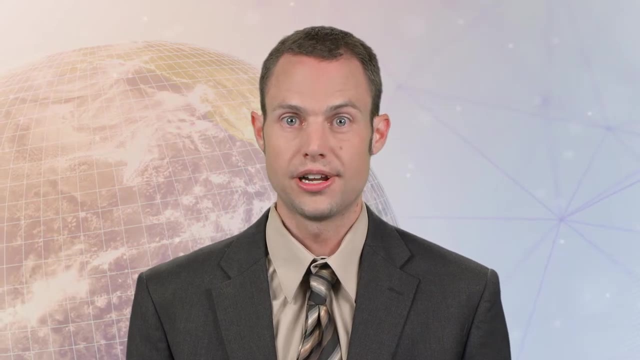 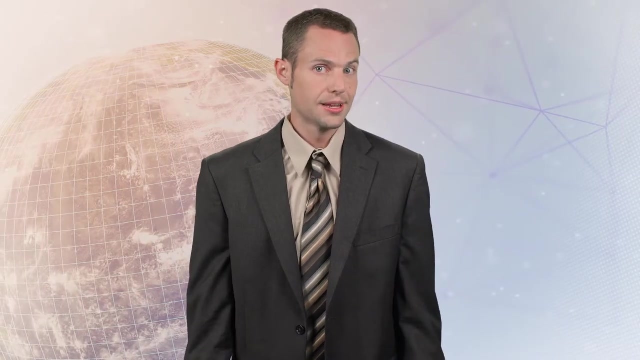 or about 23 feet. That would significantly flood coastal cities around the world, such as Hong Kong or Miami, with profound impacts for the 634 million people currently living in low-lying coastal zones, While melting sea ice will not impact the sea level, 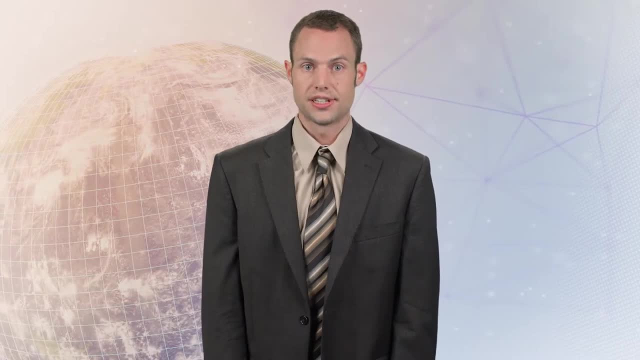 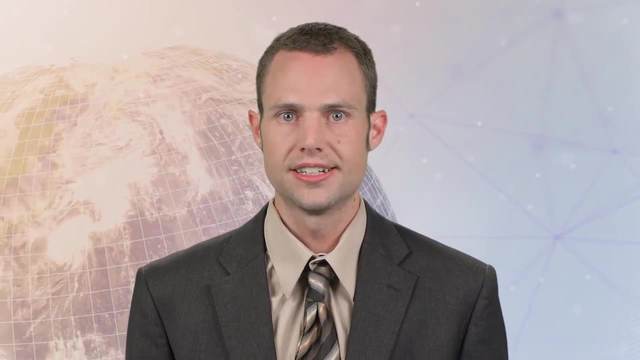 it can certainly have an impact on the atmospheric weather patterns. today, Sea ice traps heat in the ocean, so as warmer water flows into the Arctic Ocean from the Atlantic and Pacific Oceans, the heat does not escape into the atmosphere. Normally, this allows cold air masses. to form over the Arctic, which often causes the Arctic Ocean to collapse. So as warmer water flows into the Arctic Ocean from the Atlantic and Pacific Oceans, the heat does not escape into the atmosphere. Normally, this allows cold air masses to form over the Arctic. 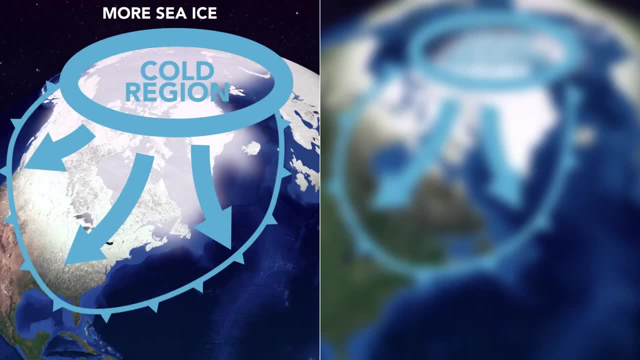 which often causes the Arctic Ocean to collapse. So as warmer water flows into the Arctic Ocean from the Atlantic and Pacific Oceans, the heat does not escape into the atmosphere. thought often becomes stronger throughout the winter, But when the ice melts in the summer. 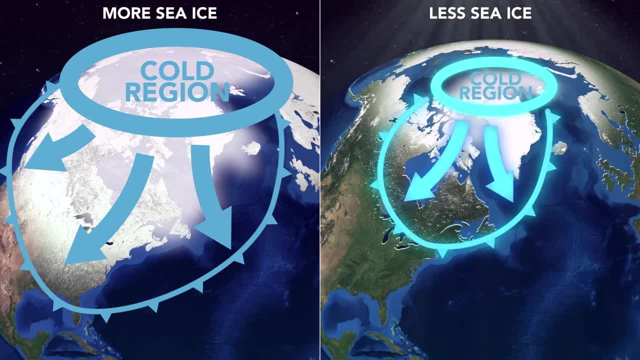 it drastically reduces the region over which cold air masses can develop, and the cold fronts that bring Arctic air into the United States are no longer as strong because there isn't as much cold air to bring out of the Arctic The ice albedo positive feedback loop. 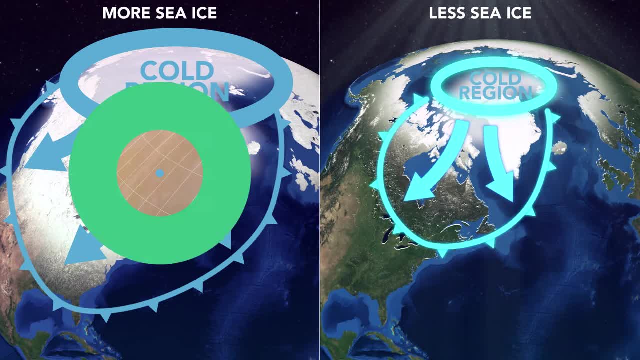 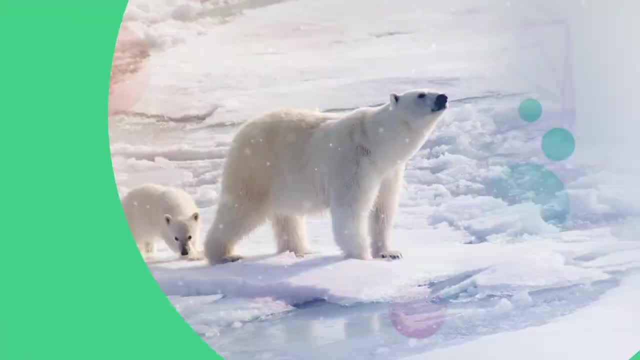 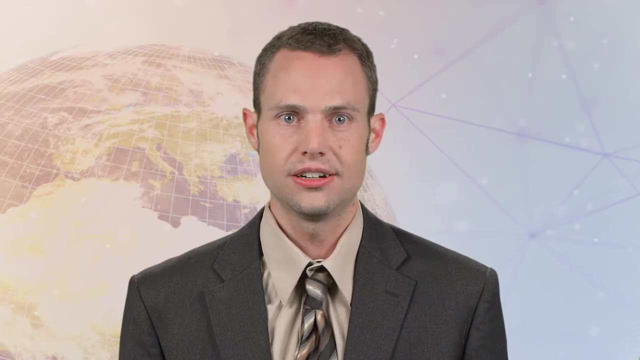 has direct consequences for people and ecosystems. Declining annual ice extent exposes land to coastal erosion, affecting Inuit communities. Biologists are observing changes and eating patterns of iconic Arctic species such as polar bears and seals. The shifting or feeding habits and species ranges impact subsistence hunting.